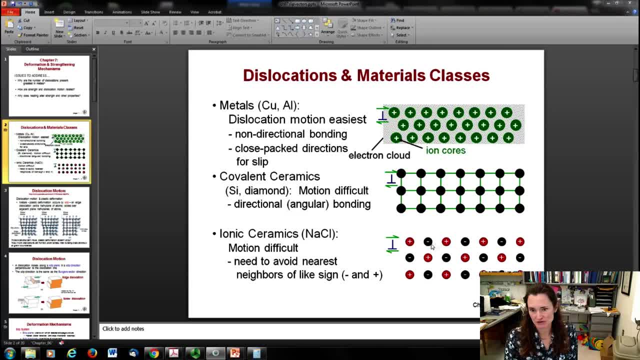 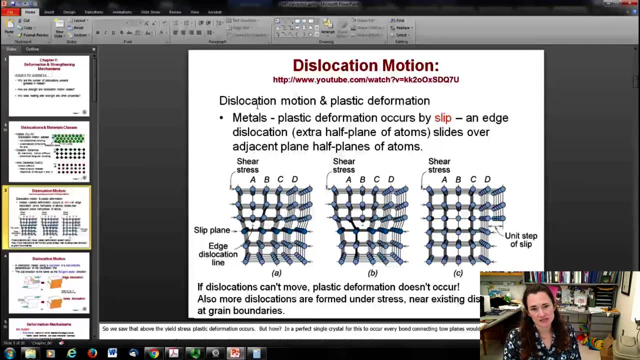 or at least pass through it, And it really doesn't want to do that because then it would be surrounded- It's nearest neighbors- by positive charges and not negative charges, and that's not very favorable, okay. So what happens is the dislocation motion occurs when things are plastically deformed. 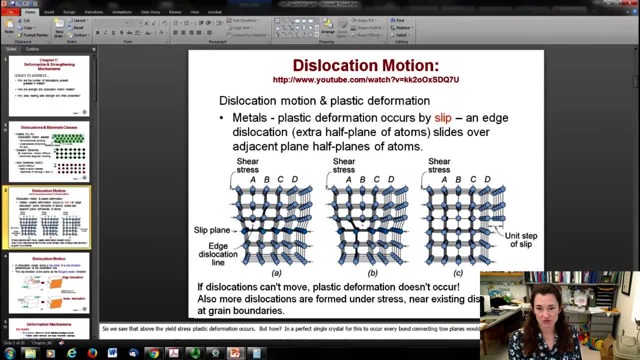 Plastic deformation occurs by slip, when an edge dislocation, which is that extra half plane of atoms slides over an adjacent half plane of atoms. So here you can kind of see a still frame version of that. Remember that, Okay. So this little symbol right here, this little T upside down T, the red thing here is a. 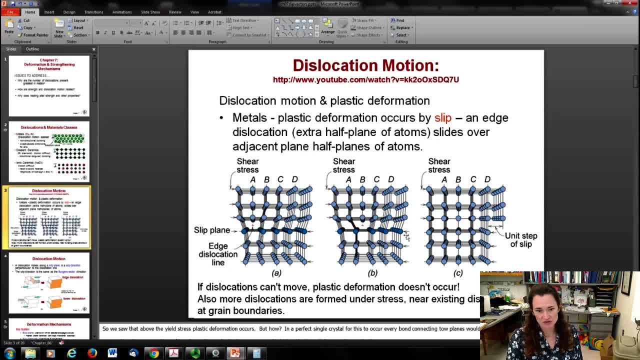 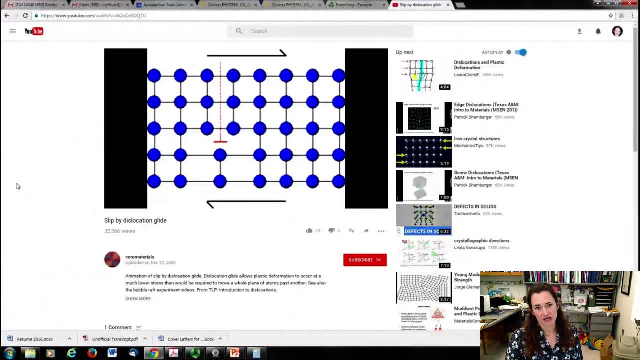 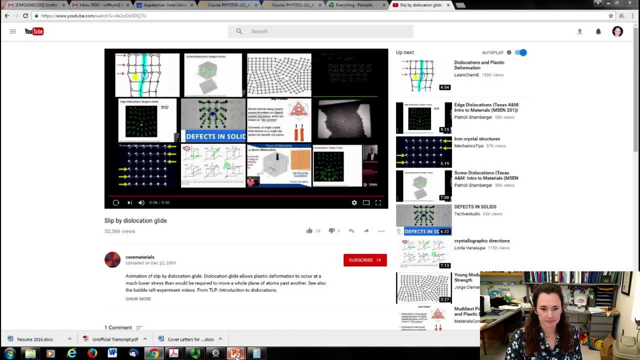 symbol for an edge- dislocation- and it just kind of moves through. I have a little movie to show you of that that I'll show you real quick. So here is that dislocation moving through the material. It's just a real simple little movie, but that's kind of what you see. 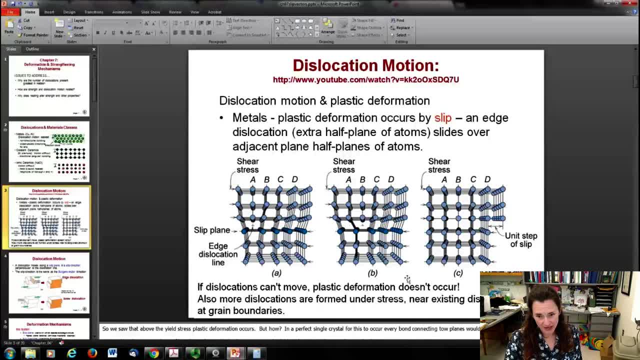 Okay, If the dislocations can't move, then you can't get plastic deformation and it just does not occur. Also, the dislocations are going to be formed generally under stress and they're going to happen near existing dislocations or at the grain boundaries. 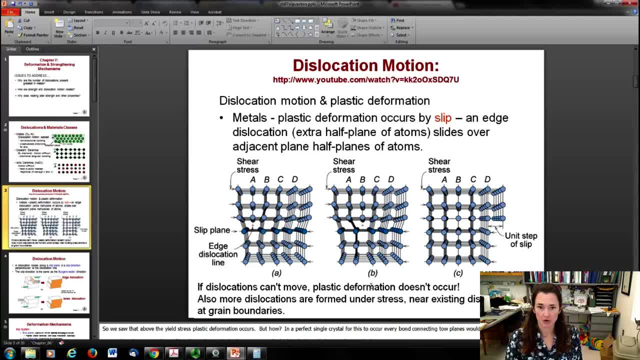 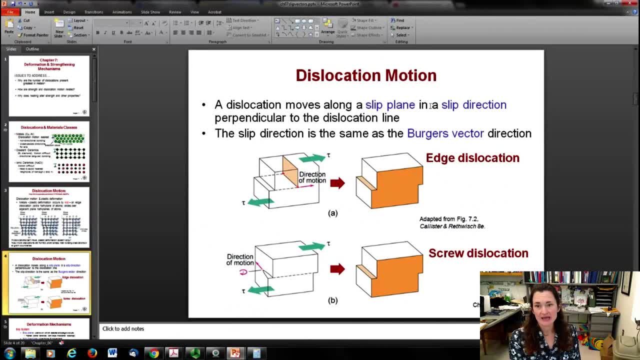 That's where it's going to start. It's going to start at the grain boundary and move through. okay, So the dislocation is going to move along a slip plane in a certain plane, in a slip direction. okay, And that will be. the slip direction will be perpendicular to the dislocation line. 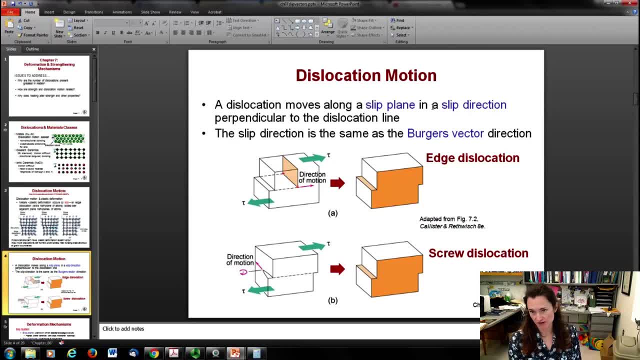 And the slip direction is the same as the volume. Okay, So that's going to be the burgers vector direction. okay, So basically, here's a little cartoon of that. You have your shear stress applied here and then it causes the dislocation to move along. 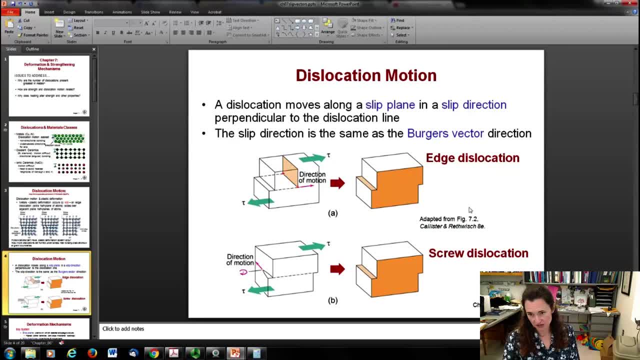 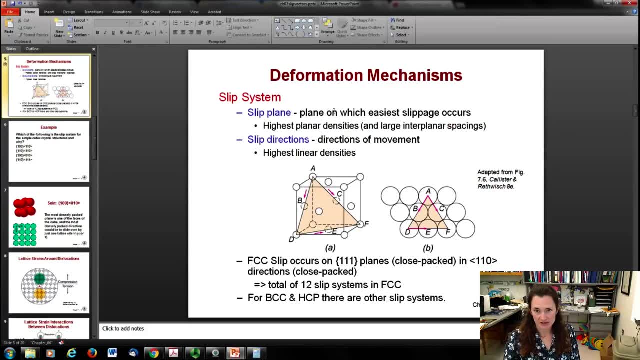 a certain plane in a direction. Okay. so there's your edge, there's your screw: dislocation. So which directions are these? Well, your slip planes are going to be the planes on which the easiest slippage occurs, And those are going to be the ones with the highest plane. 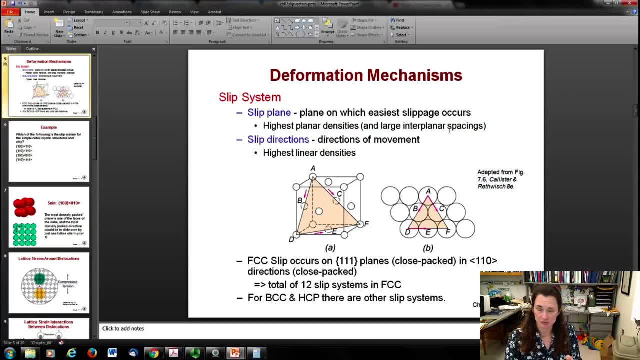 And those are going to be the ones with the highest linear densities and large interplanar spacings, And the slip directions, those directions of movement are going to be the ones with the highest linear densities. And it chooses the highest density direction because, remember, you're having atoms hopping. 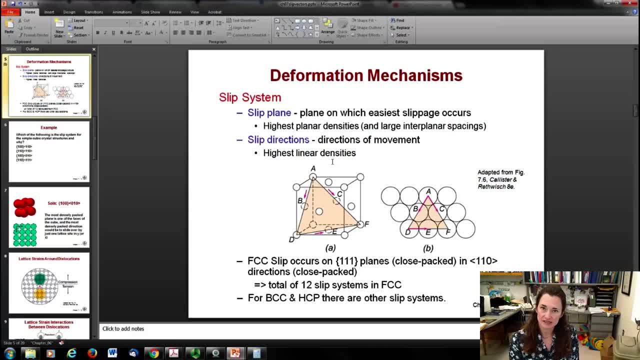 from one position to another, And the directions with the highest densities are going to be the ones where hopping from one lattice position to another isn't very far. okay, So here's a little cartoon of an FCC map. Okay, So that's the material. okay. 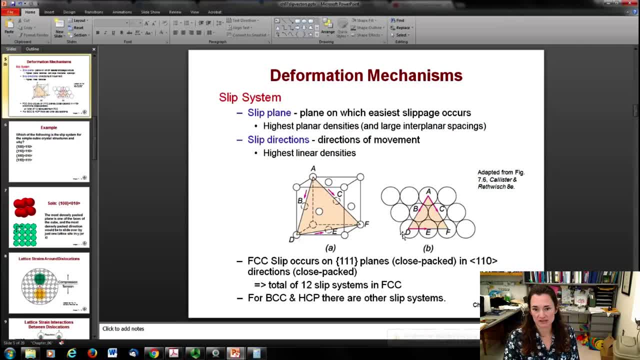 And the slip plane is going to be along the 111 because that's the tightest packed. That slip plane here is shown in this sort of orange colored triangle And then here's a 2D view of that, So you can see that's a very highly packed direction. 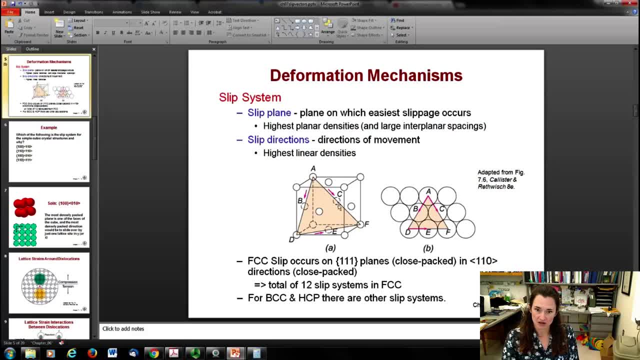 So here's A in the upper back corner, B is along the face, and so is C, it's along the back face, And there's DEF and that shows you the little cartoon. Okay, so that's the slip plane. it's a very high density plane. 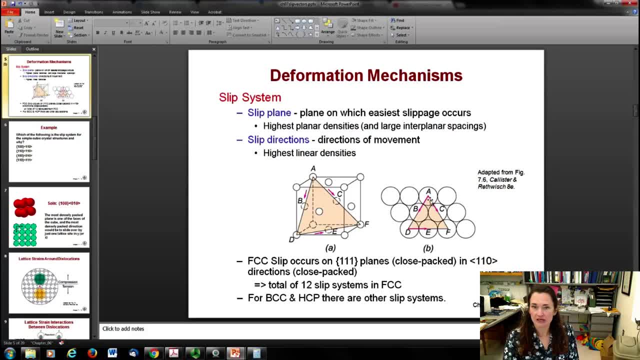 And then the slip directions are going to be along any one of these directions, where it just has to hop to its nearest neighbor to move across. So that'll be sort of a family of directions along A, B, A, C or from D to E. okay, 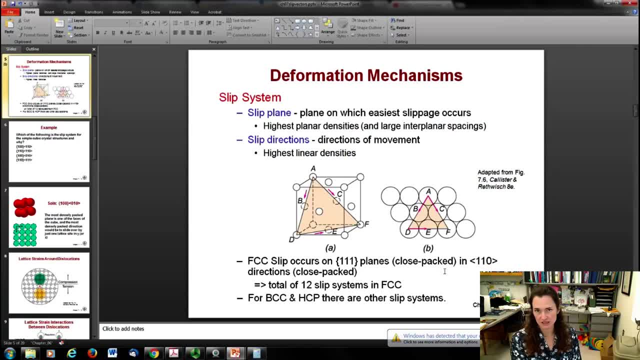 And so there's going to be a total. there'll be more multiple slip systems in any given crystal. For FCC, that's 12 slip systems, And in BCC or a hexagonal closed packed, it'll be different directions, but it's the same. 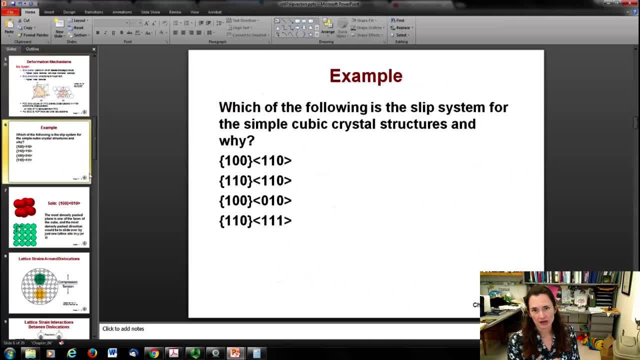 concept. So an example: which of the following is the slip system for a simple cubic structure, and why? Okay, so your choices are, you know, the 100 family of planes along the 110 direction or the 110 family of planes along the 110 direction. 100 family of planes along the. 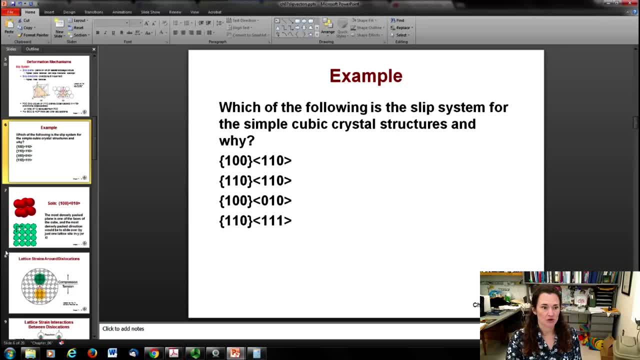 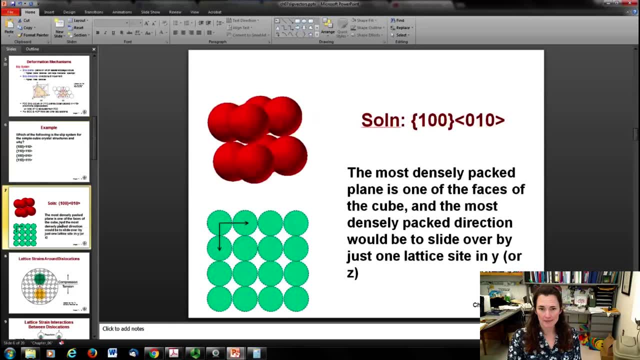 010 direction, and so on and so forth. okay, So the solution is that it's going to be this one right here, this 100 family of planes along the 110 direction. Why? Okay, well, if you remember what a simple cubic system looks like, it's just a little. 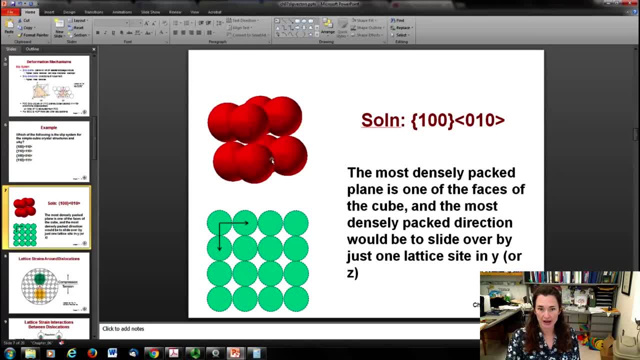 cube with an atom sitting at each of the corners. okay, So the tightest, highest density plane is going to be along any one of the faces of the cube. That's the highest density. So I've shown that here in a little cartoon in a 2D view. 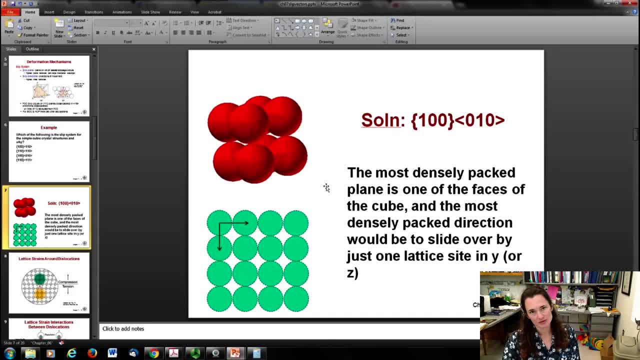 If you cut across the diagonals, for example, that's not going to be as high density because there's a larger distance in between the corners. There's a larger distance in between the corners of the cube than there is along one of the faces. 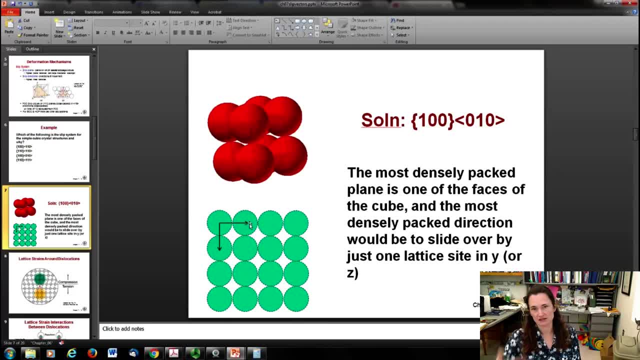 So here's a cartoon picture of one of the faces in sort of a multiple cube stacking. So that's the family, So it's the 100 family of planes, and then it's going to hop also nearest neighbors. It's going to hop from center to center this way. 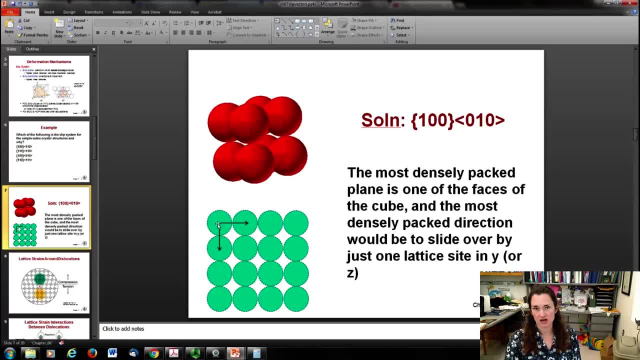 If it hops along a diagonal, that's a further distance and so it's not as tightly packed, And so that corresponds to the 010 family of directions. okay, It's going to hop this way, this way, It's going to hop this way. 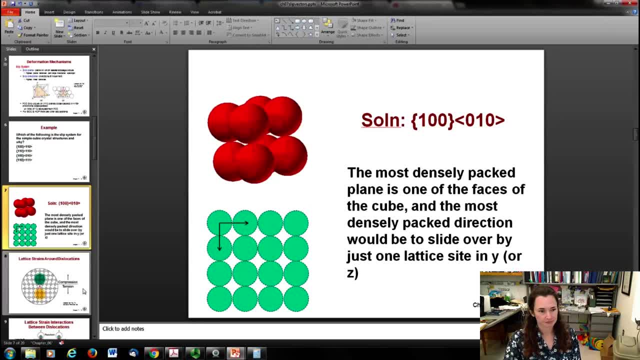 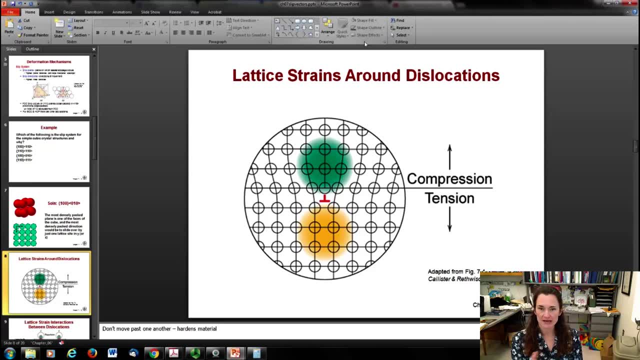 It's going to hop, even in z and that'll be the direction chosen. Okay, so what happens is, as you move that line of edge dislocation through, you're going to have a region of compression and a region of tension. okay. 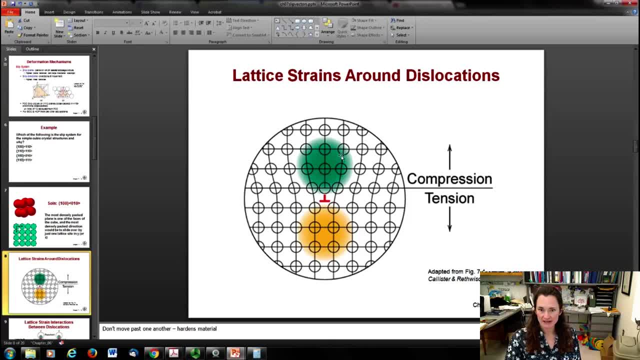 The compression is going to be where the lattice is a little more tightly packed than it would like to be. Then it will feel a compression, It will feel a strain in one direction and the tension will be. the lattice is a little further apart than it would like to be, So it's under tension there. Okay, So there's a strain. 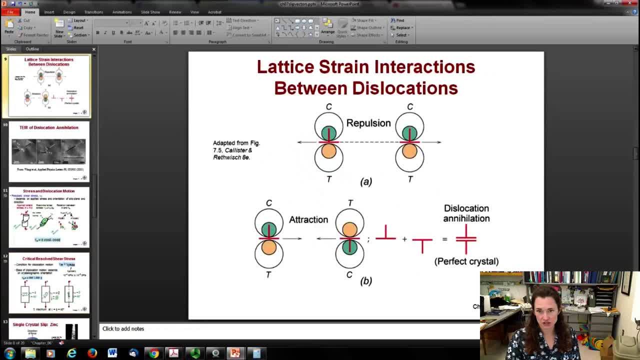 a strain in the lattice around any given dislocation. Now what happens is, as these things move through the material like strains, repel one another right. So if you've already got a compression, it doesn't want to move towards another compression because that would. 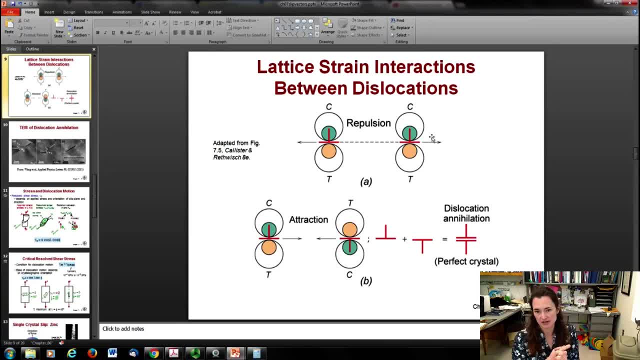 create even more compression and too much stress in the lattice. So what happens is you get these likes repelling. However, uh, unlikes. if a compression sees a tension, it wants to move towards that, and that'll relieve the stress and hence lower the energy state of the system. And 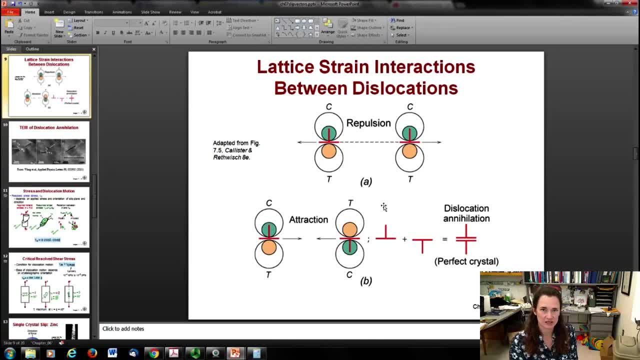 when that happens, they annihilate. So it's kind of a similar idea to positive and negative charges. right, When they move together, the net charge is zero. When a compression and a tension move towards one another, the strain goes away, And so that's what happens and you get a perfect crystal. 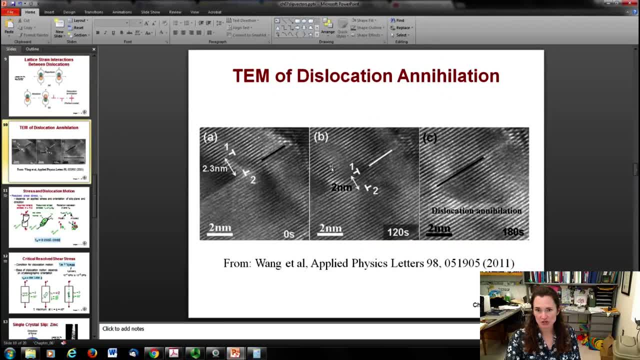 there. Um, this was actually captured in a little TEM movie and I here I show you some still frames from the movie, from an applied physics letters paper in 2011.. Remember, TEM is transmission electron microscopy, And so if you stare real hard at this for a little while, you can see two. 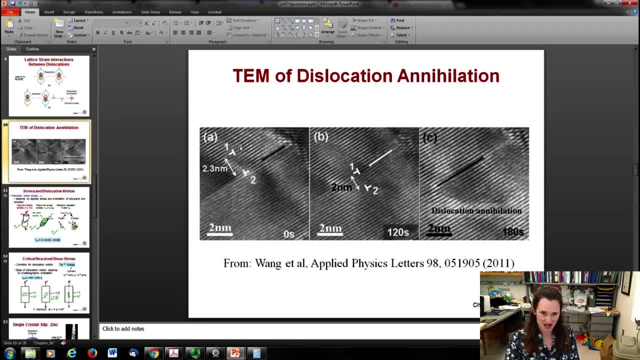 edge dislocations- and they've labeled them here for the ease of the eye for one and two- And they initially started out about 2.3 nanometers apart, but over time, as they took the movie, these dislocations got closer and closer together until they annihilated and became a perfect crystal. So 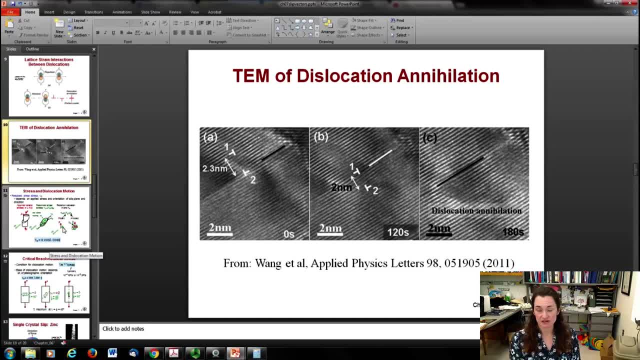 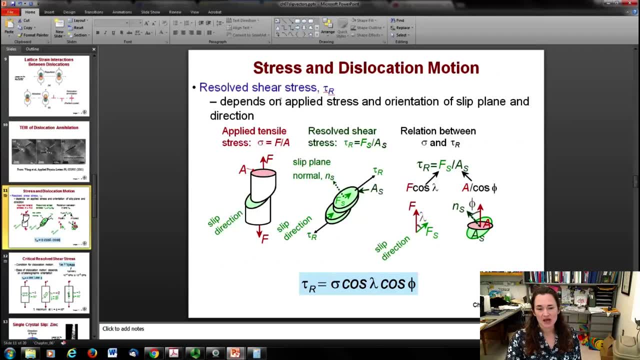 we're able to these days, not just talk about this in a theoretical way, but actually image it and see it happening, which is pretty exciting, Okay, Um, another important concept to understand is the idea of a resolved shear stress and how that affects the dislocation motion. So let's say that. 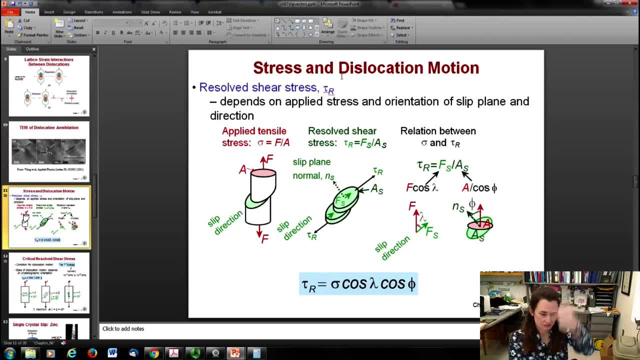 you've put your bar or whatever one of those tensile testing machines and you're giving it a pull. Okay, Now the thing is, your slip direction, um, is going to occur along a direction that might not necessarily be aligned with the direction of the force that you're applying to the material. Okay, And so what'll happen is you'll 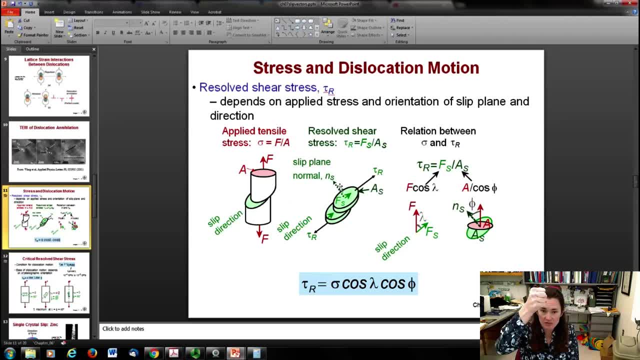 have a force, um, but then that will not be aligned with the shear force, the shear direction for the plane. Okay, Um, so you're going to have to resolve the shear stress. Only a portion of that force that you apply will go into causing slip. Okay, So how are those two? 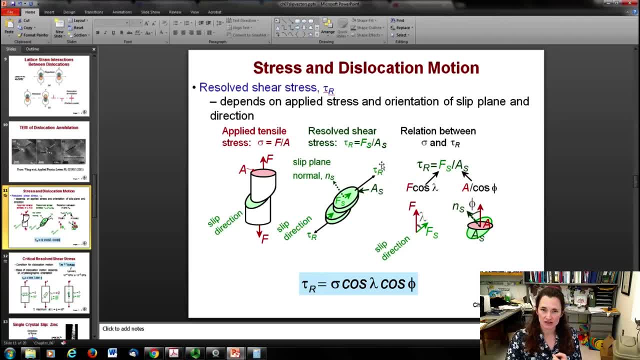 things related. Um well, basically the, you've got the dot product that you're going to take for the direction of the force applied to the direction of the force that is sheared right. So you're going to resolve the force applied to the. 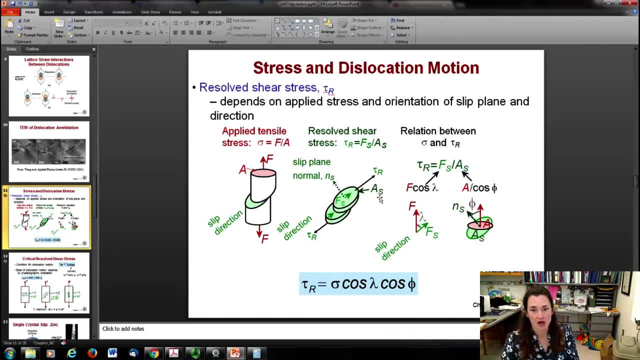 shear force, which is actually what causes the slippage Um. so there's one dot product there where you're going to take the dot product of the applied force To the shear force direction And the angle in between those two things is called lambda. Okay, So that's your slip direction versus your applied force. And then you're going to have to resolve the direction between your um- shear stress- and the slip direction. Okay, And the angle there is phi, So that's the angle in between your slip um direction and your applied force. All right, So your critically resolved shear stress. 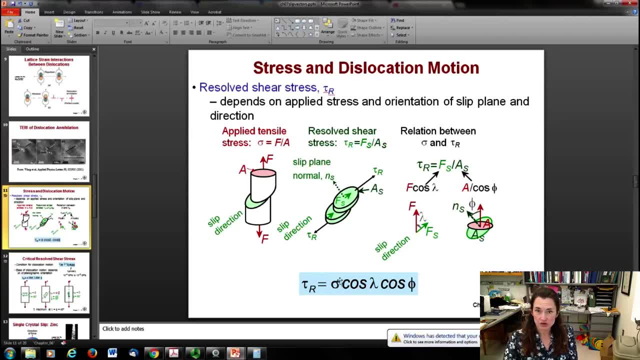 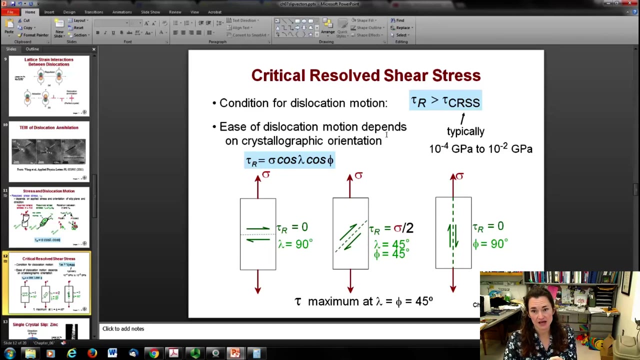 tau sub r is going to be the shear stress that you apply from your load machine times the cosine of these two angles, um, between the direction uh of the applied force and the slip plane, and the slip direction, phi and lambda. Okay, So the condition for a dislocation to move is that your resolved shear stress has to be greater than what's called the critically resolved shear stress. 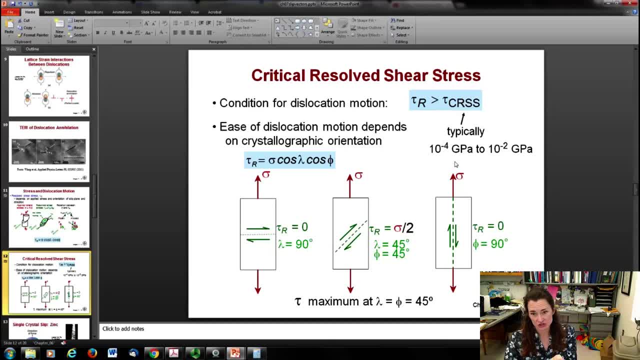 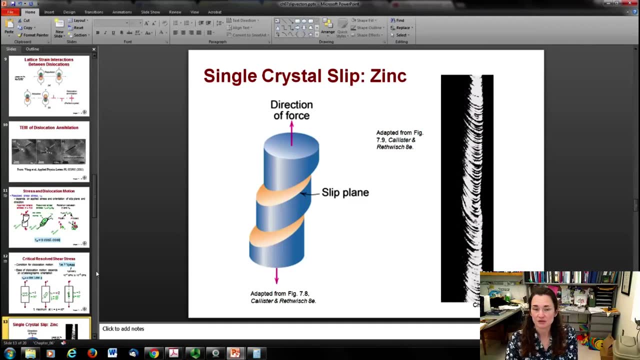 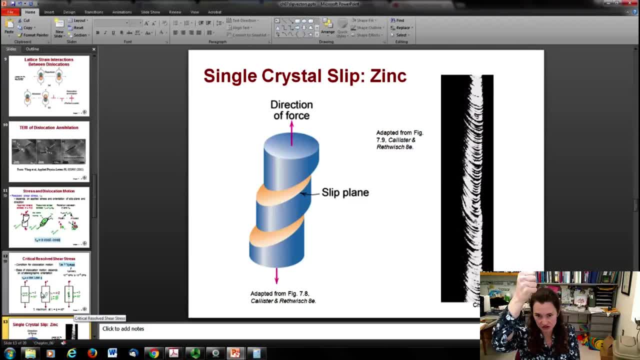 And so the slip planes were not aligned, of course, with the direction of the tensile stress, And so you see these little directions of the slippage, And because it is a beautiful single crystal, then that turned into this kind of gorgeous looking little slip plane stair step thing where it's slipping right along the direction of the shear stress. So that's fun. 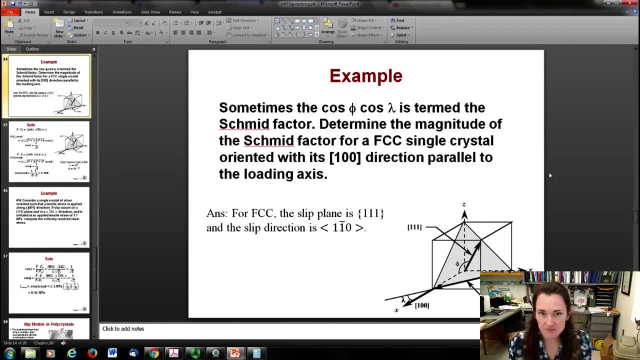 Okay, Let me do a couple example problems here. Sometimes they call the cosines of those two angles phi and lambda Repetition, And so that's why it's called fcc, FCC, single crystal that's oriented with its 100 direction parallel to the loading axis. 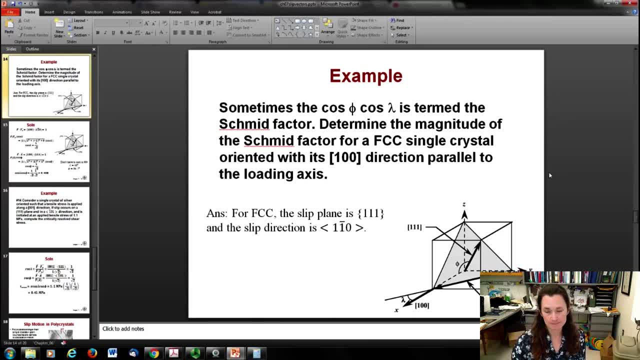 So that's the direction that it wants to slip in Now. remember we already talked about the FCC family of slip planes and slip directions. So for FCC, the slip plane is in the 111, it's the 111 direction that's the most densely. 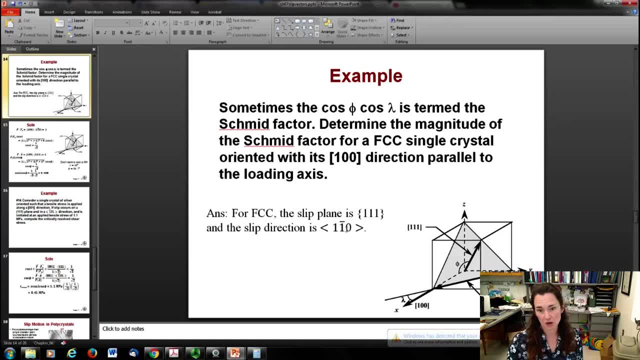 packed plane And the slip direction is going to be the 11 bar O direction. okay, so that's the direction it's going to want to move between the most tightly packed direction. Remember, for that you've got your, your, your atom here at the corner, your atom here. 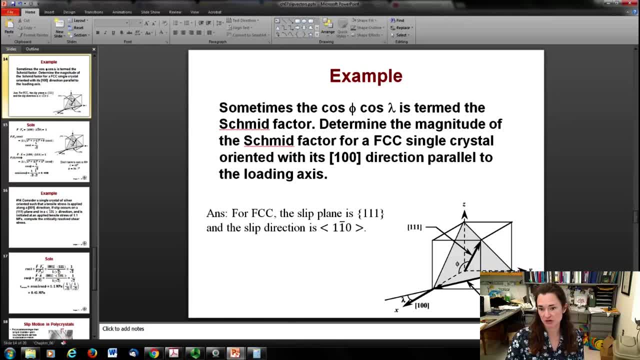 at the center and your atom here at the bottom, So that's the most tightly packed direction. it's going to want to slip along that direction. So it's going to slip along this plane and kind of that way, pointing in the direction of lambda. 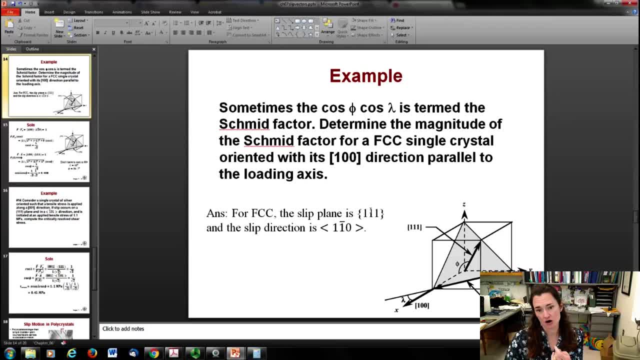 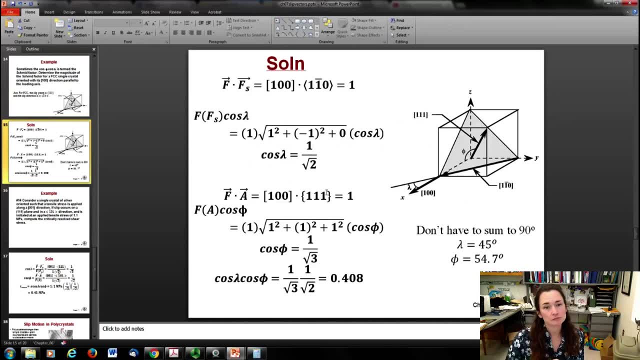 So we need to resolve this. okay, for our slip plane slip directions and the direction of our load, that's being applied. So let's take some documents, Dot products: okay, The force applied to the shear force will be the dot product of the 100 direction that. 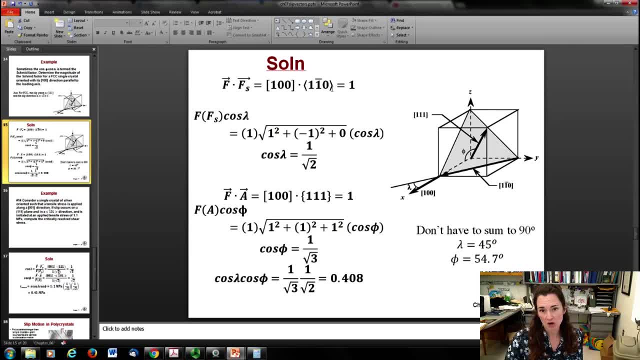 the force is applied in with the slip direction: 11 bar O. okay, And when you take that dot product you get one times one plus zero times minus one plus zero times zero and that gives you one. So that's your dot product. 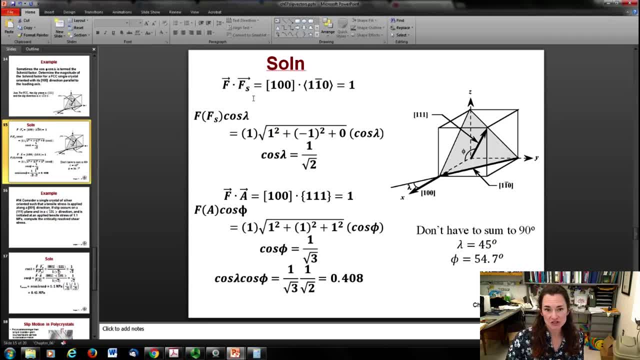 And now that dot product. if you set the magnitude of the dot product, it would be equal to the magnitude of the force times the magnitude of the shear force. Okay, So the magnitude of this 100 vector is the square root of one squared plus zero squared. 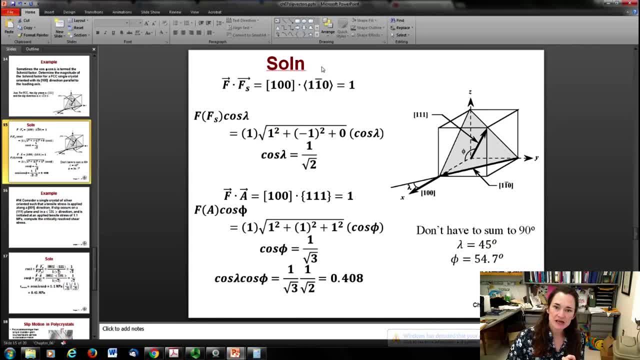 plus zero squared. Of course, that's one, it's a unit vector. And then the next is the magnitude of this vector, the one one bar O, and that's the square root of one squared plus minus one squared plus zero. So that gives you the square root of two. and then times cosine lambda. 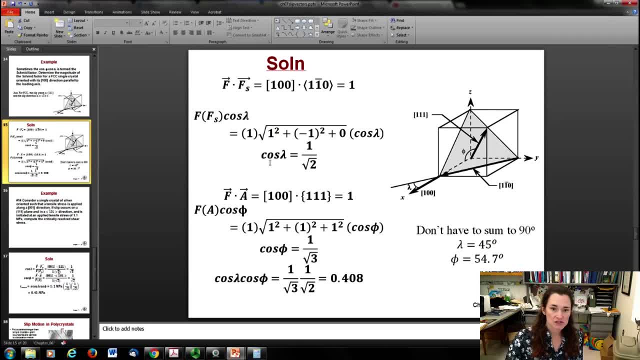 And lambda cosine lambda is what we're trying to solve for. So, cosine lambda: if you set this dot product, Dot product equal to the magnitude of the dot product, and solve for lambda cosine lambda, you would get cosine lambda is equal to one over the square root of two. okay, 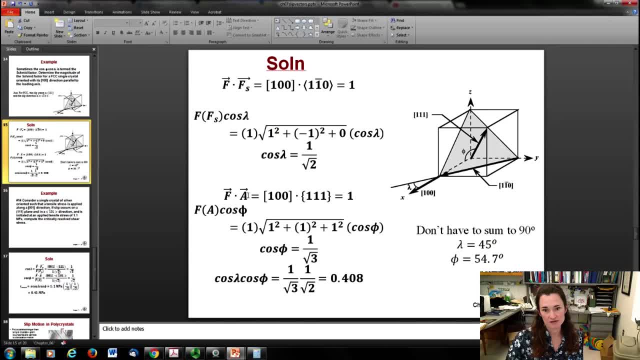 That's part of it Now. the other is the dot product of the family of plane with the applied force. So there you're doing the dot product of the one O O direction for the loading with the one one, one family of plane, And so when you do that you've got one times one plus zero times one plus zero times one. 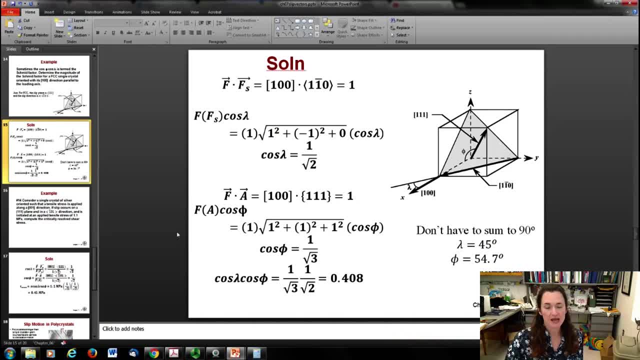 again and you get one. So that's the total dot product. The magnitude of that dot product would be the magnitude of the force, vector times the magnitude of that area, vector times the cosine of phi, which is the angle there. So yet again, the magnitude of the force is one because it's a unit vector. 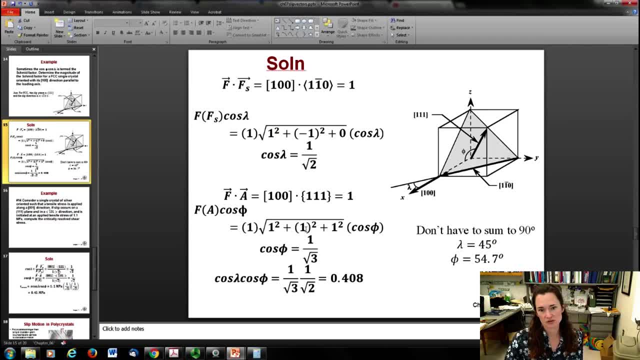 And for the one one one, it's the square root of one squared plus one squared plus one squared. So that gives you the square root of three, and then times cosine of phi. Okay, And then solving for cosine of phi, You get: cosine of phi is equal to one over one. 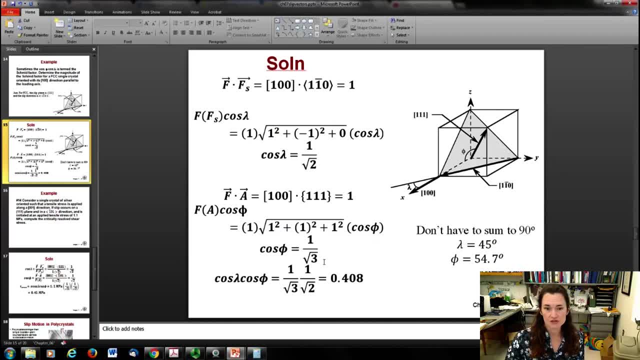 Okay, It's equal to one over the square root of three. So your Schmidt factor is cosine lambda times cosine phi, which is one over root three times one over root two. And if you figure out, plug that into your calculator, you get 0.408.. 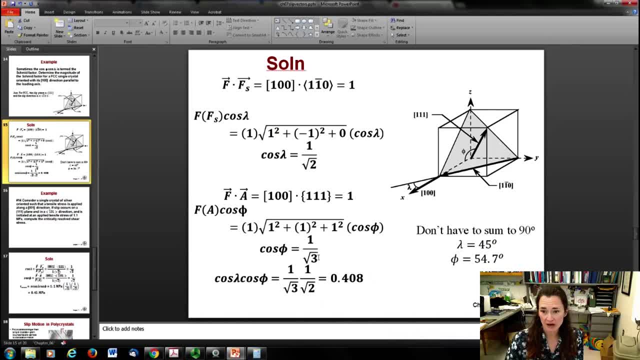 So that's your Schmidt factor. Now I want to point out that your direction for your, your value for your slip plane and your slip direction- they don't have to be perpendicular to one another, because that's something that a lot of people do. 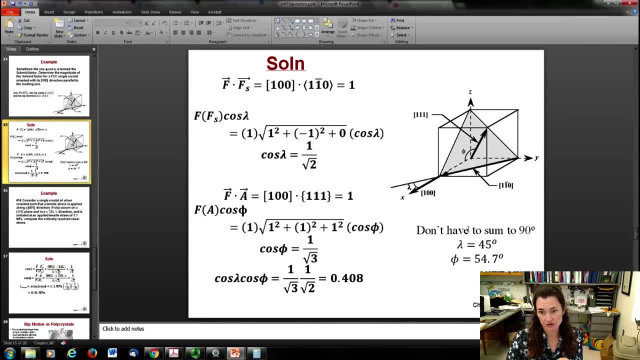 Kind of think is true, but they don't have to sum to 90 degrees those two angles. If you solve using inverse cosine of lambda is equal to inverse cosine of one over root two, then you get lambdas equal to 45 degrees, but solving for a five you get 54.7 degrees. 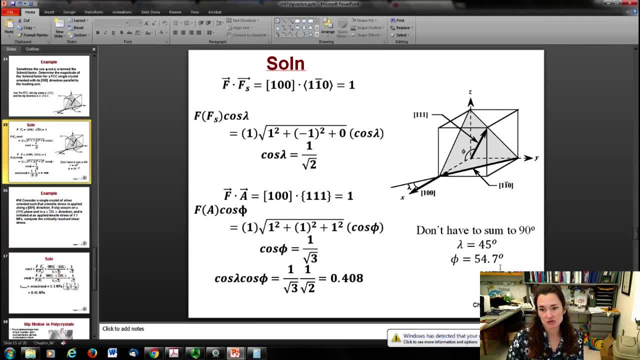 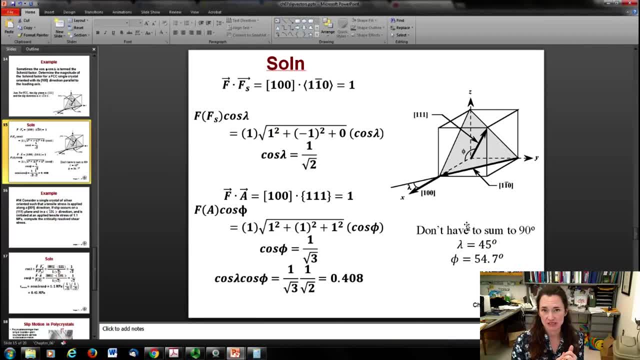 And that is true, For example, for that simple cubic example that we did a little bit ago: the 1 0, 0 family of planes and the 0 1, 0 slip direction. those are perpendicular to one another. So it can happen, but it doesn't have to happen. 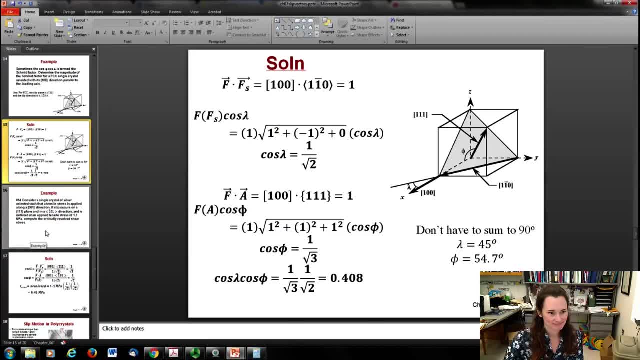 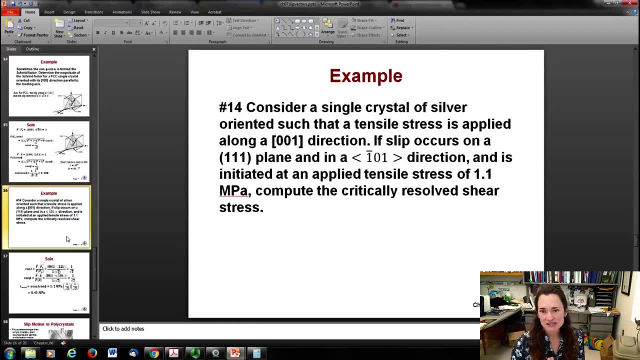 If that makes sense, Okay. Okay. Next example, Cause I think all this work is worth repeating: Consider a single crystal of silver oriented such that a tensile stress is applied along the 001 direction. Now, if slip occurs in a 111 plane and in a 1 bar 01 direction and is initiated, 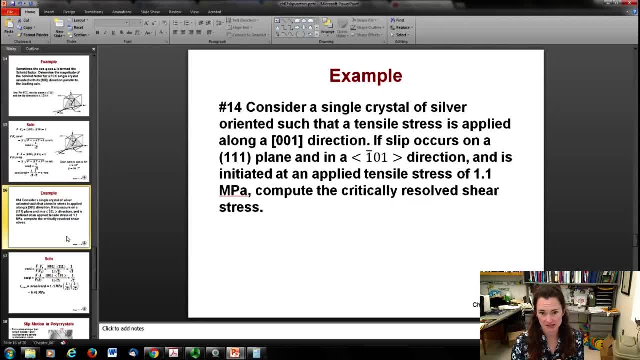 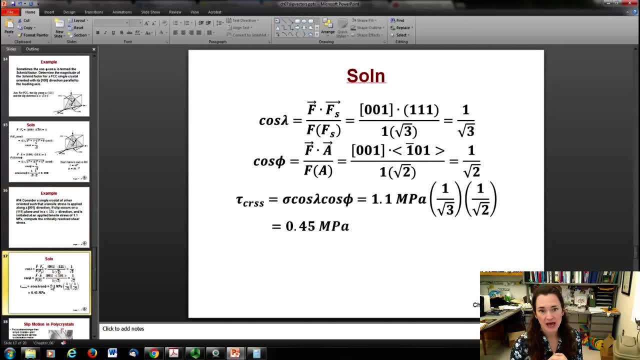 at an applied tensile stress of 1.1 megapascals, compute the critically resolved shear stress. okay, So here we have. we're going to solve for our cosine lambda and cosine phi, again in a very similar way to the way that we did before. So we're going to do the dot product of the 001. 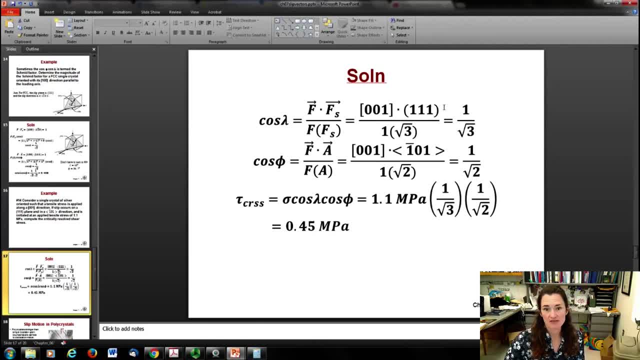 direction with the 111 plane, and then divide that by the magnitudes of those two vectors to get our cosine lambda, and that gives us 1 over root 3.. And then for phi, we're going to do the dot products of our 001 direction with the 1 bar 01 slip direction, and that gives us 1 over square root. 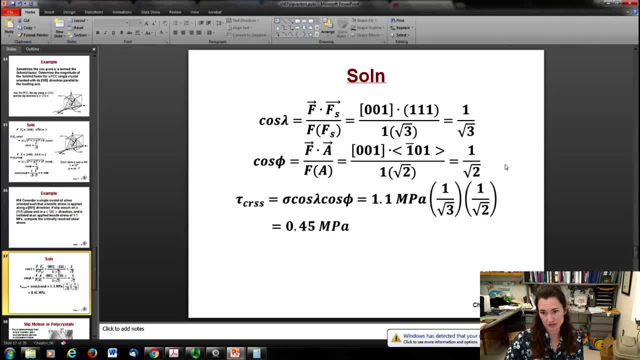 of 2.. So our Schmitt factor is yet again 1 over root, 3 times 1 over root, 2.. Now to compute the critically resolved shear stress you're going to do the dot product of our 001 direction with. 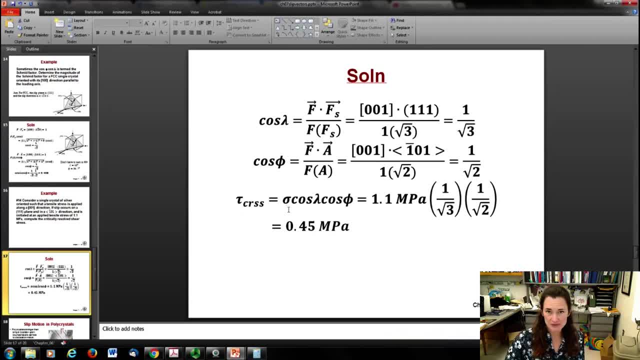 the 0.4.. So you're going to multiply your stress at which slip is initiated, which was given to you in the problem as 1.1 megapascals, and then you're going to multiply that times your Schmitt factor. 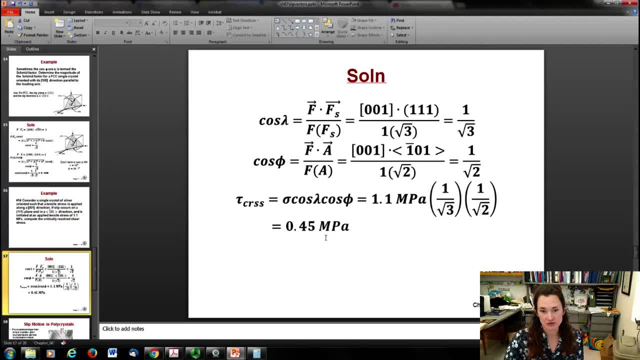 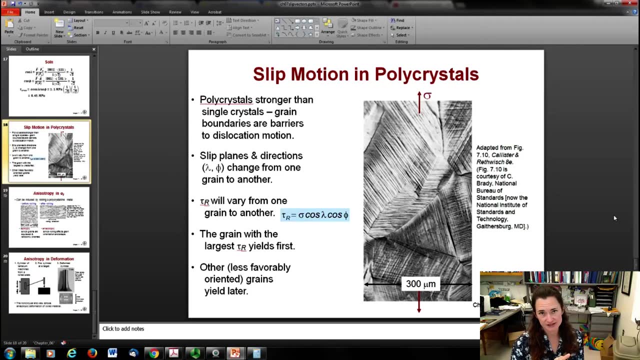 which is 0.408, just like it was before. And when you do that you get a critically resolved shear stress of 0.45 megapascals. okay Now, single crystals are rare. It's actually quite difficult to get a single crystal of material. It takes a long time. 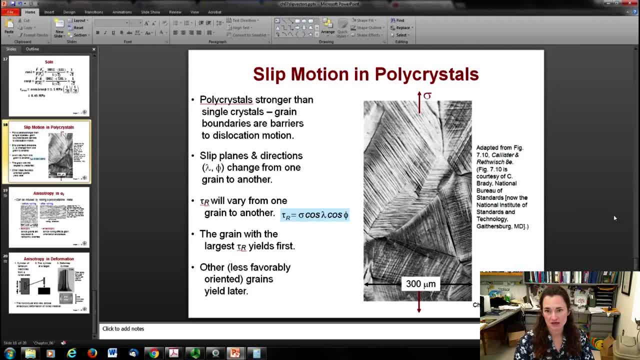 and it takes a lot of effort. What's more common is, of course, a polycrystalline material. okay Now, in a polycrystalline material, they have a tendency to be stronger than single crystals. 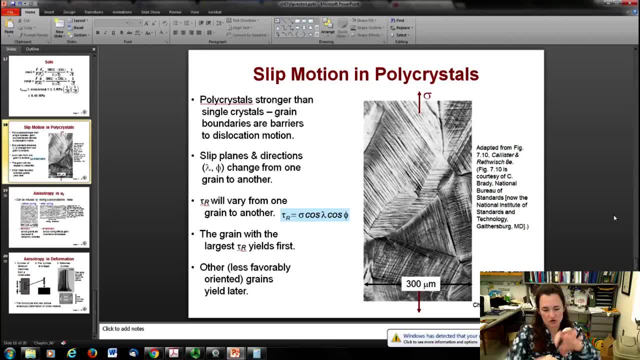 and the reason is that the crystals, the domains, are oriented in all kinds of crazy ways right, So they don't necessarily line up. So those grain boundaries become barriers to the motion of the dislocation, Like let's say that you have one and the slip direction is this way and it's going. 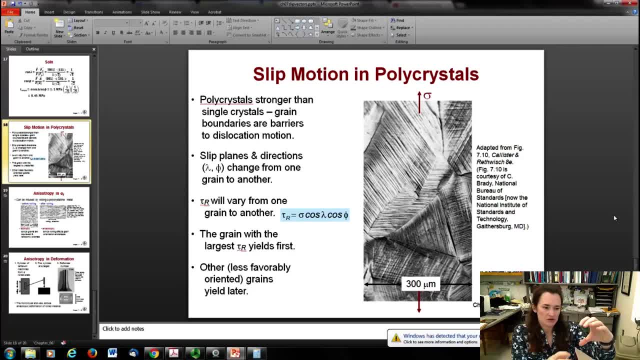 this way, but in this one it's kind of okay, well, those aren't in the same direction, So it's slipping this way and it comes to the edge and it's trying to make it slip this way and then it just stops. okay, So a polycrystalline material. 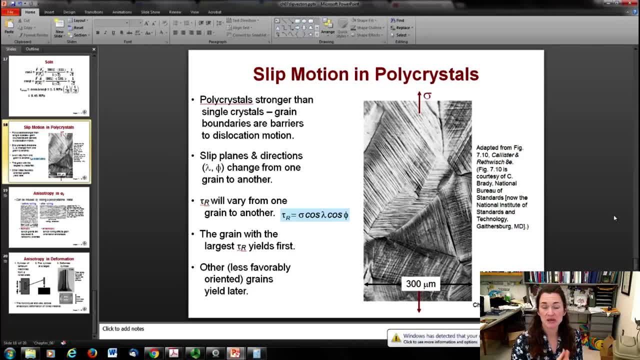 is stronger and tougher than a single crystal material because those slip planes and directions change as you go from one grain to the other. So that means that your resolved shear stress is going to vary from one grain to another. So what's going to happen is you're going to apply. 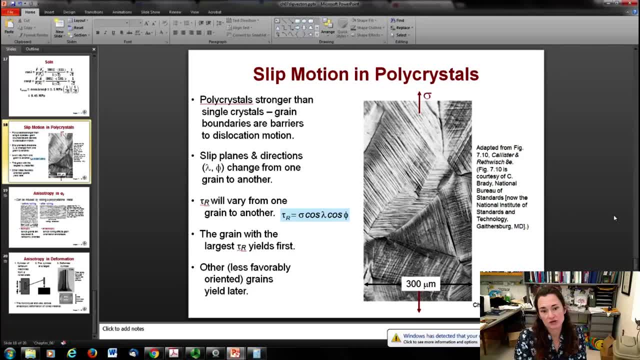 a shearyou're going to apply a stress and the grain with the largest resolves. your stress will yield first, but then the others maybe won't yield as much. okay, So that results in sort of a resistance of the material and it'll stop and it won't deform as much that way. 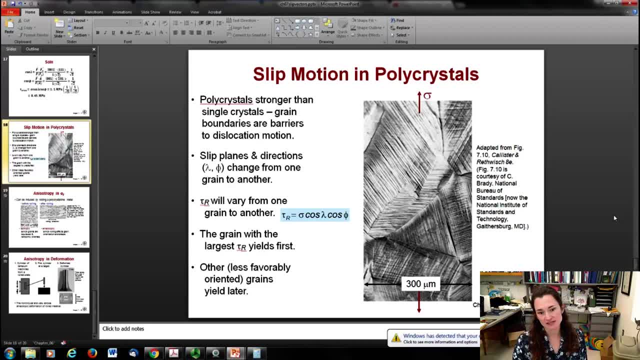 That makes the whole thing stronger, And the other, less favorably oriented grains will yield at a larger applied force, if that makes sense. okay, So you're getting more of a resistance to the force when you have that Now, this SEM image right here. 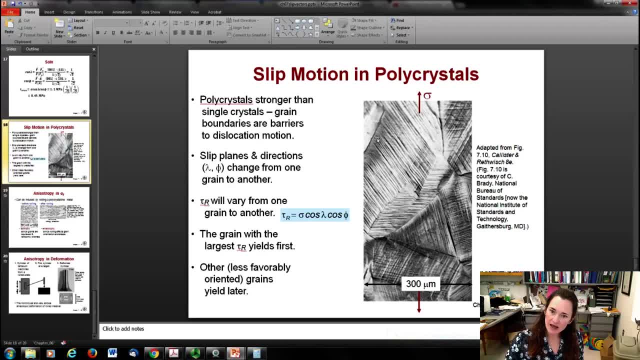 shows you some of these dislocations. These lines in the SEM image are the dislocations that have occurred. This thing has been applied, a stress has been applied, and then you can see that the slippage is in different directions, along different grains. okay, 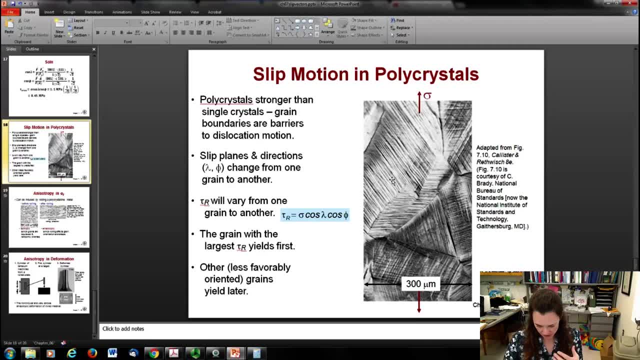 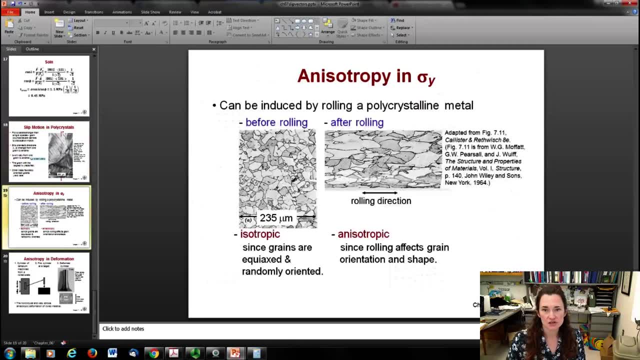 And that shows up in this SEM image, So you can see that the slip directions are different as you go from domain domain. you can also get anisotropy in a material and you might want that sometimes, depending upon your part, if you roll out your metal in a certain 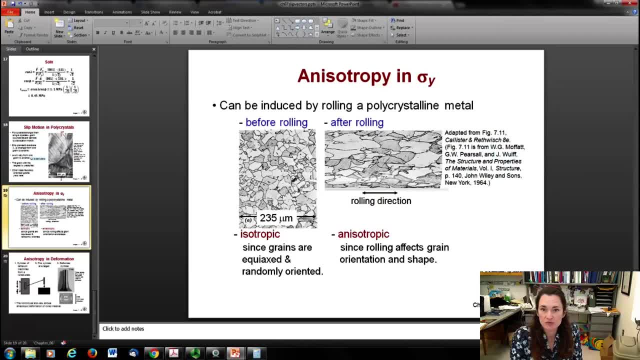 direction. that'll stretch it out in a certain direction and that'll make your grains not symmetric. okay, so this is an image of some isotropic grains in a material before it was rolled out and then, after you roll it out, that in causes the grains to be elongated in the direction of rolling and it's an. 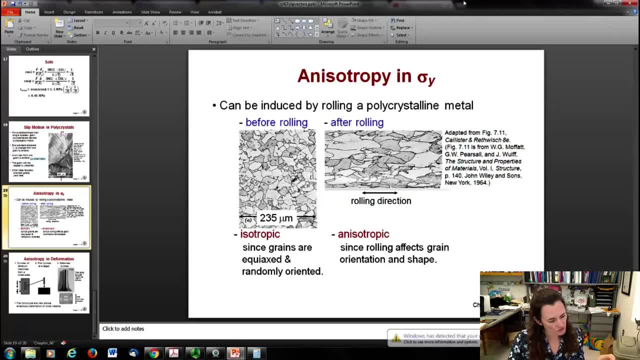 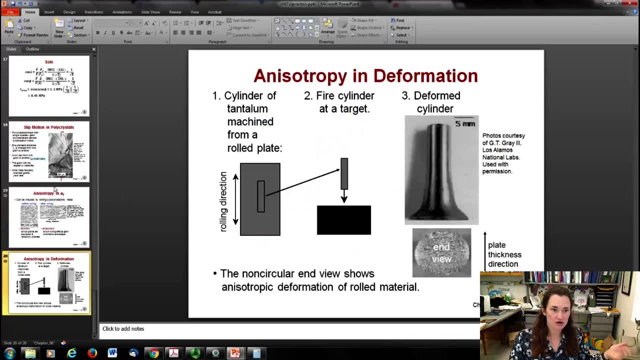 anisotropic material then. so what means is that under stress the boundaries are maintained, but the whole grain is going to elongate in the direction of the applied force, and that can cause some anisotropy in the deformation. so here they took a material that had been rolled out in a certain direction. they